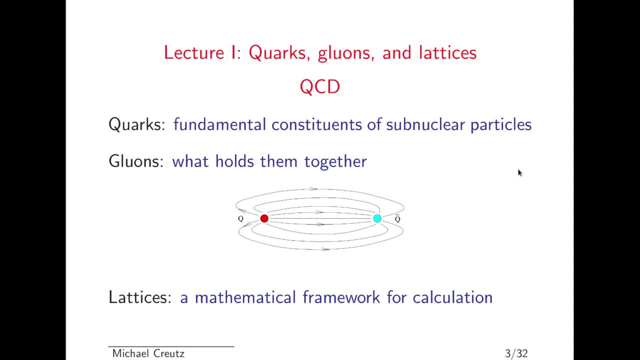 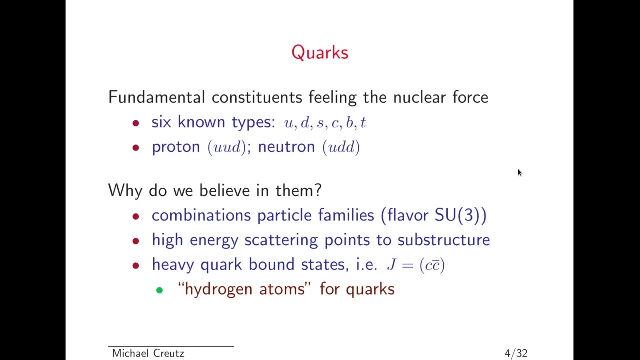 fundamental constituents of the sub-sub-nuclear particles. The gluons are the fields that hold them together And the lattice approach is a mathematical framework in order to calculate things with quarks and gluons. Now, the quarks, as I said, are the fundamental constituents that feel. 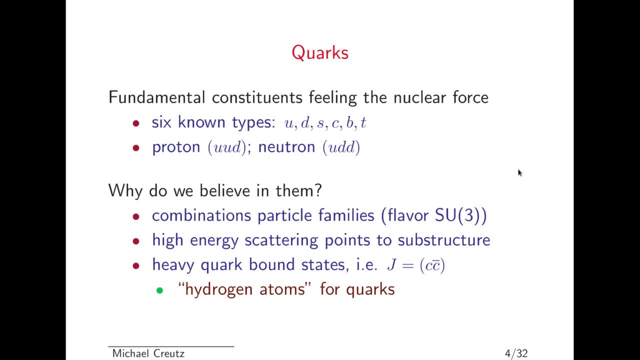 the nuclear force. There are six known types: U, D, S, charm, bottom and top. Proton is two up quarks and a down bound together. Neutron is an up quark and two down quarks bound together. So why do we believe in quarks at all? Well, first of all, 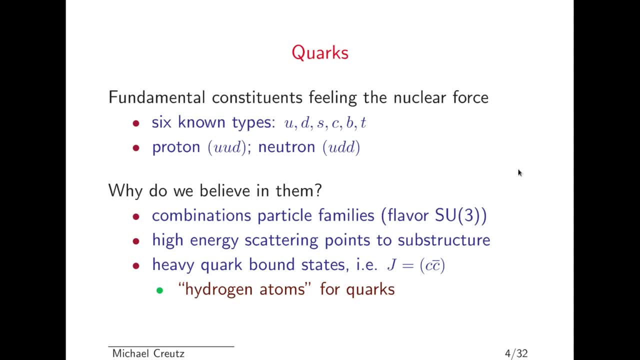 different combinations of them generate particle families. In particular, you see that the proton and the neutron are related to each other. just by changing the flavors of the quarks in there, Uh, another reason to believe in quarks is that, uh, high energy scattering experiments basically started as slack show for of electrons off of protons First of all, show the proton has. 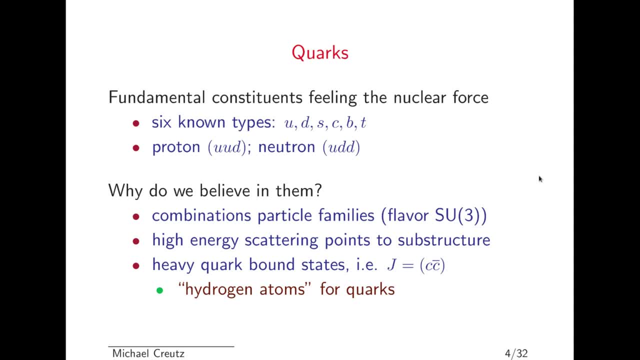 a finite size by 10 minus 13 centimeters. But when you hit it really hard, occasionally electrons comes flying off at a very wide angle, which is kind of like shooting a gun in a paper bag and all of a sudden something ricochet out of there. So there's something hard in there. 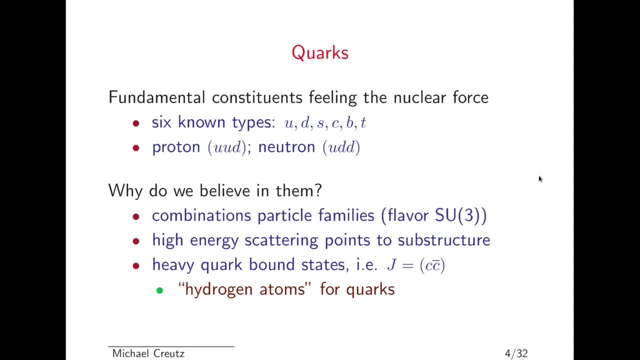 Uh then, the next reason to believe in quarks really appeared when they discovered the heavier quark bound states such as the JMS. This, uh, the heavier quarks don't move as fast, and so you can actually treat them approximately non-relativistically, And so these are sometimes. 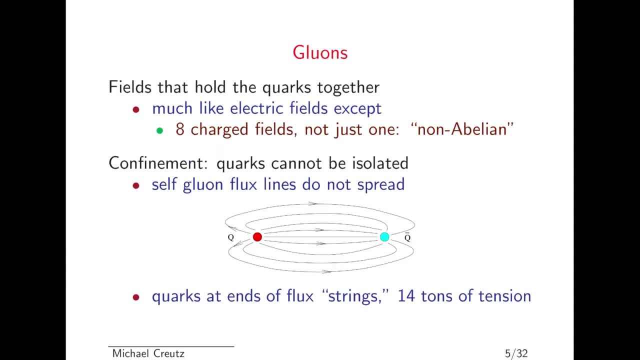 thought of as the hydrogen atoms for quarks. The gluons are the fields that hold the quarks together. They're very much like electric fields with one and the other. They're very much like electric fields with one and the other. They're. 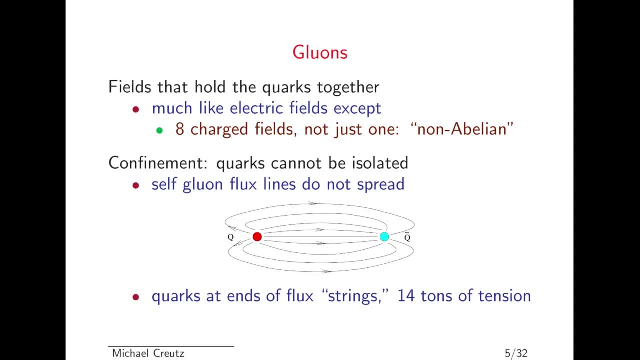 an exception. They're charged. They're charged with respect to each other. There's not just one, There are eight of them, and they've satisfied what's called a non-abelian symmetry. Now, confinement is an interesting property of this game. 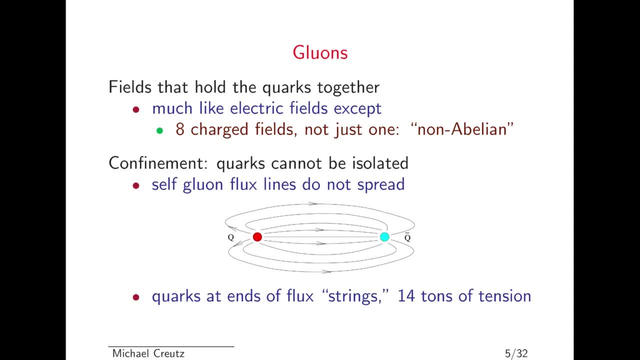 The quarks apparently cannot be isolated. They've never been found alone. They're always in their bound states And the idea why this occurs is that the gluon flux lines come out of a quark, They try to spread out. when the flux lines come out of a quark, They try to 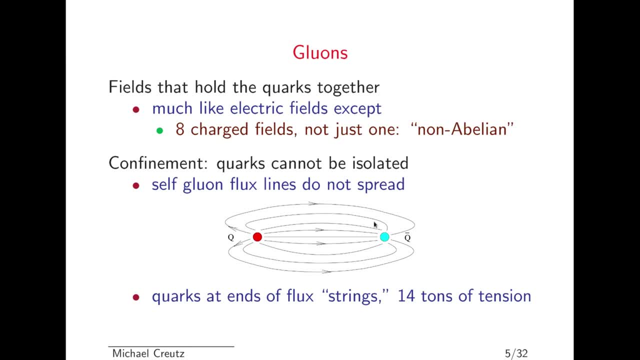 spread out, but they're attracted to each other and they go on together until they find the anti-quark And they generate what is effectively a flux tube between the quarks and the anti-quarks. And the quarks are the ends of the strings These strings have. 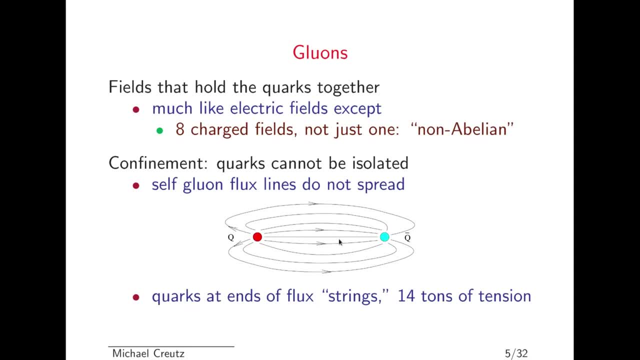 empirically about 14 tons of tension. So it's huge, Huge. So confinement is kind of like the reason you can't have a string with only one end. Of course protons are like strings with three ends and that comes out of the group theory. 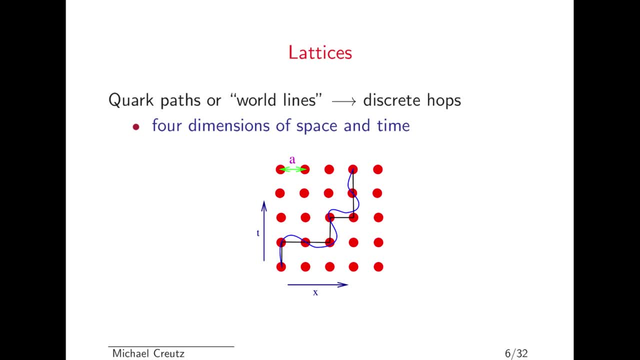 Okay. so the lattice's starting idea here is to replace the paths that a quark can take through space-time by a sequence of discrete hops. And it's a four-dimensional system because we discretize both time and space. And the idea is: this is a mathematical trick. 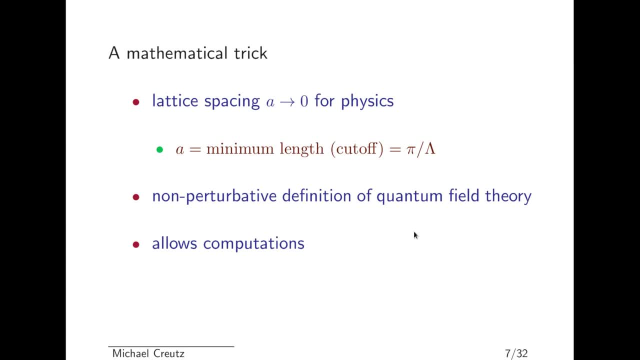 What we want to do is take the lattice spacing smaller and smaller for real physics, because it's just a, it's basically a cutoff, It's a minimum length, Or you can think of it as pi divided by a maximum momentum. Now, this does a couple of good things for us. One: it gives us a non-perturbative definition. 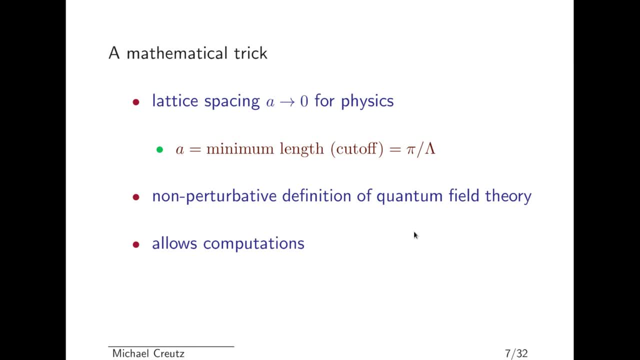 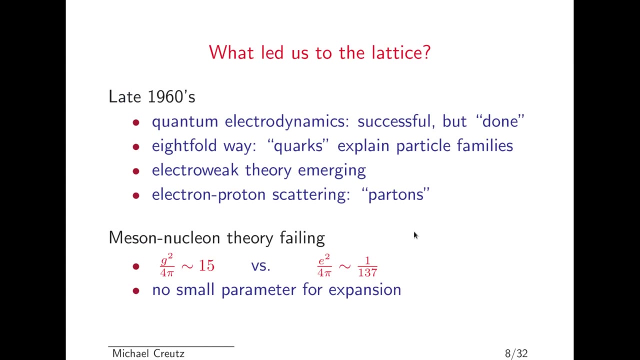 of quantum filtering. Quantum filter is the continuum limit of this system, And the other nice thing- which will be a lot of the school- is it allows one to do computations. So why did we come to this strange, peculiar way to treat space and time? 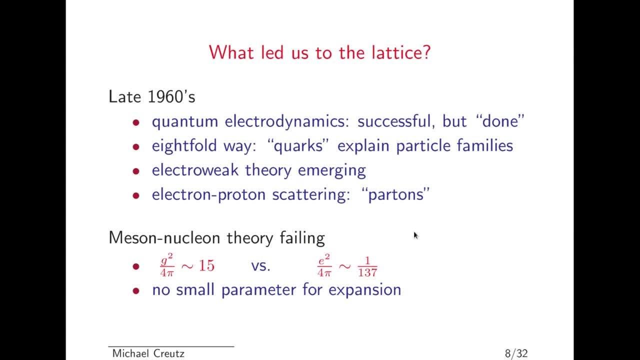 Well, in the late 60s, when I was a grad student, quantum electric dynamics was very successful as a field theory, But in some sense it was done. We knew all the principles of it. The calculations got harder and harder but we sort of knew how it worked. This was also a time. 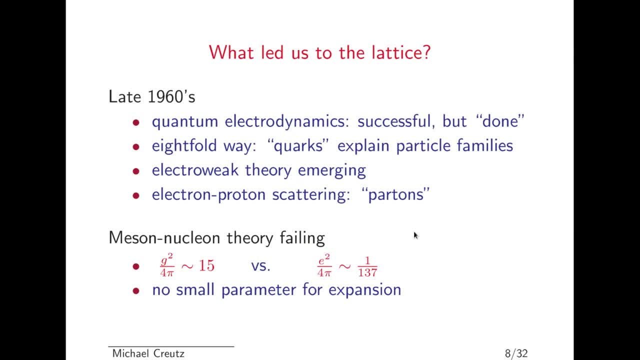 of the eightfold wave, People were finding families of particles and quarks. very nicely explained the families they found. This was the time when the electric weak theory was just beginning to emerge. Then there was this exciting stuff of the electron-proton scattering, where 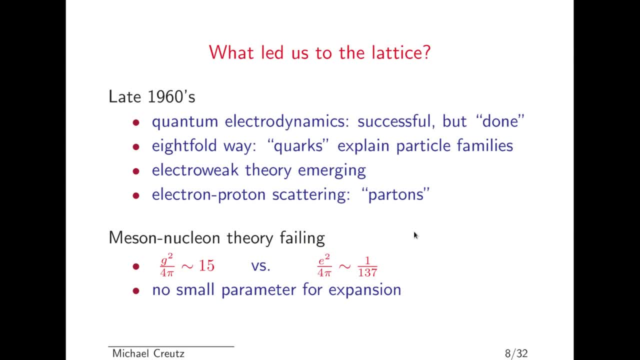 these hard things inside the proton were called partons. At the time nobody dared identify quarks with partons, although later on they became realized to be the same thing. But at this time there was a theory of mesons interacting with nucleons which was failing miserably The 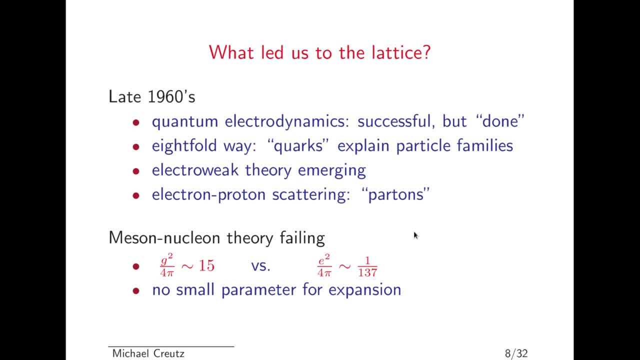 coupling constant was a huge number. G squared over 4 pi was 15, so when you tried to do calculations the next order was 15 times stronger versus in electrodynamics, where E squared over 4 pi is only 1 over 137.. So the problem with the meson-nucleon theory is there was no parameter. 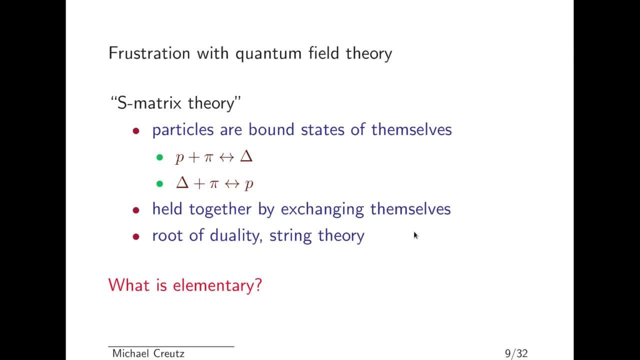 there. So there was a tremendous frustration with quantum field theory. This was a time of something called S-matrix theory, which is kind of an elegant idea which I think is a little bit too much forgotten now. But the particles could be bound states of themselves. You could take a. 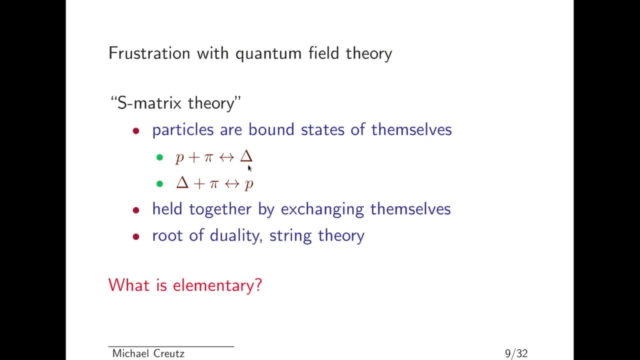 proton and a pi and bind them together and produce a delta particle. Or you could take a delta particle and combine it with a pi and produce a proton. So all the particles were supposed to be held together, but they were not held together. So you could take a proton and a pi and bind them. 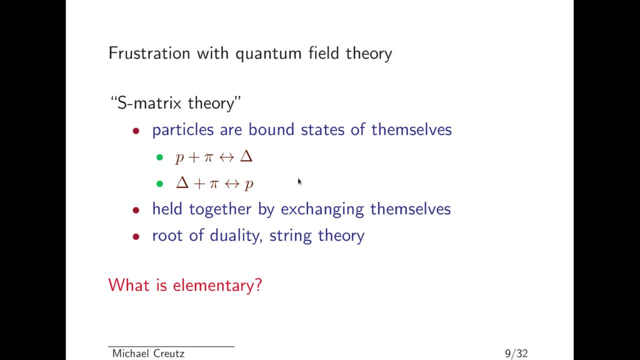 together and produce a delta particle. So all the particles were supposed to be held together, but they exchange themselves Now. this evolved over the years. This was the root of duality and is now known as string theory. But it raises an interesting question: what is elementary? Is the proton the elementary thing? 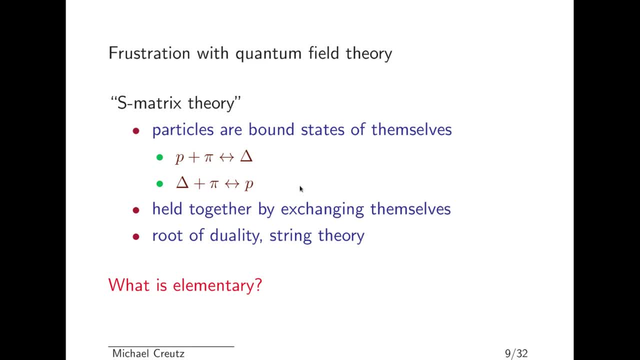 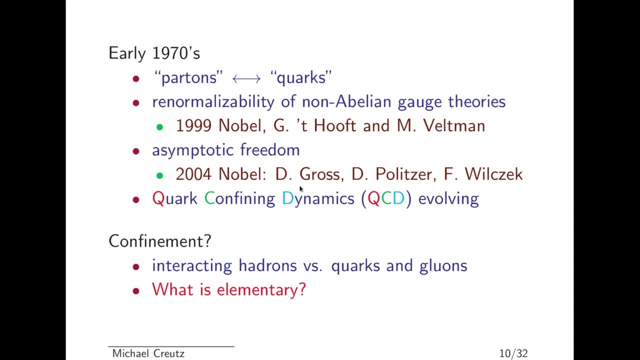 or the delta. I mean protons are a little lighter but they're both sort of comparable. Now in the early 70's people were more and more realizing that protons were the quarks. There was a couple of mathematical distinctions here, a sequence of direct Faculty use of the unknown 오. 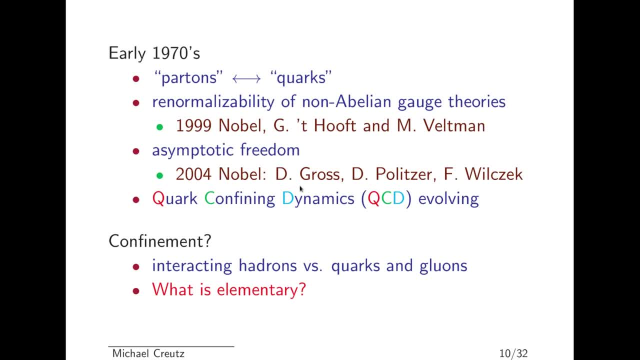 and models of dalla entry. and now electrons, the y arrow. you just don't knowTC cultural functions. So parall morality is Pokemon. you don't knowtgg with A four or a five. The one thing that I wanted was an experiment. looks like light. What my theory is going to be is something like an. 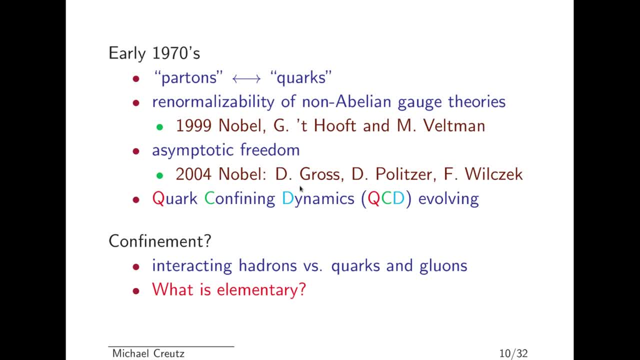 discoveries at the time. First was the non-emulant gauge series were in fact renormalizable field theories. That, of course, gave Tufton and Veltman their Nobel Prize, And it was also about this time that Grossblatt, Pulitzer and Wilczek. 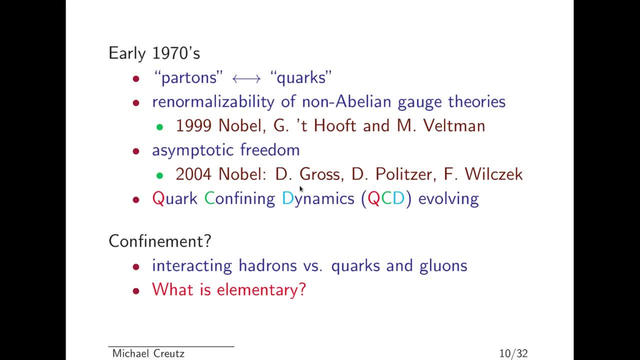 discovered this phenomenon of asymptotic freedom, that the effect of coupling in non-emulant gauge series gets weaker when the energy gets very, very high, And so these kind of things put together became QCD, the quark-confining dynamics. But the question: 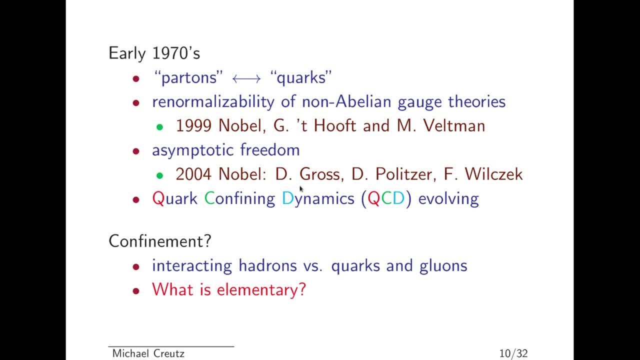 of confinement was always kind of hanging around. The basic things you saw in the laboratory were hadrons, whereas the underlying things in this theory were the quarks and the gluons. So it's again. this question arises again. what is elementary? Are the 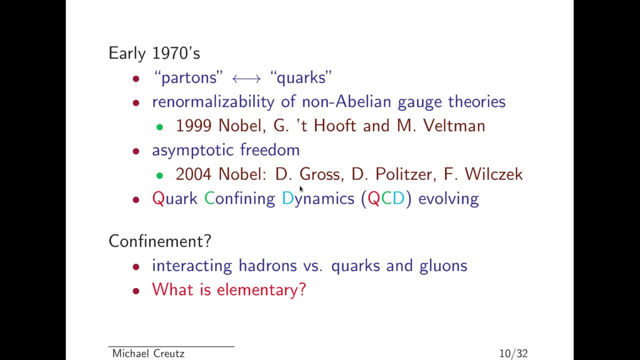 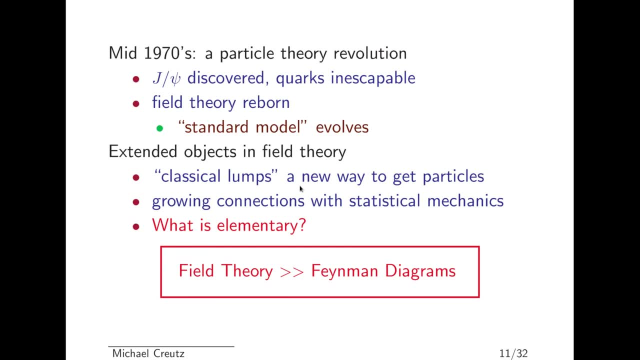 quarks and the gluons. really more elementary Are the hadrons. but they can't go anywhere, so hadrons could be more elementary. There was a big revolution in particle theory in the mid-70s. This J-psi particle was discovered. 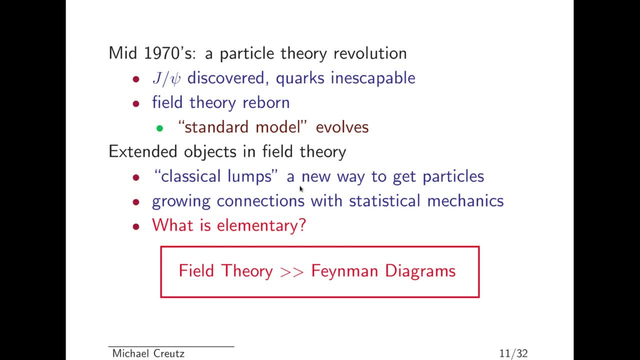 and it was very well described as a bound state of two charmed quarks or charmed and anti-charmed. So this field theory really got reborn. then We had the asymptotic freedom, we had the quarks and the standard. 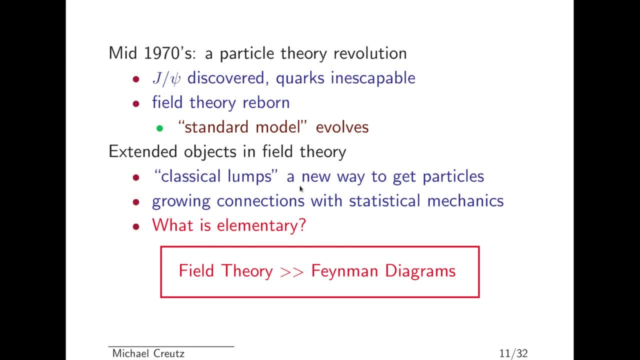 model was really evolving then. It hasn't changed in many ways since then. actually, At the time there was a very interesting set of developments. People were learning that in quantum field theory you could produce kind of extended blobs of fields which 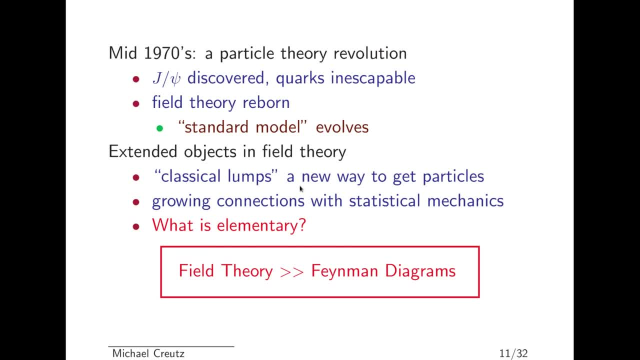 were a new way to get particles. Now. this was particularly important at the time because this was also very popular in statistical mechanics. So the connections with statistical mechanics were beginning to develop and of course, lattice gauge theory is very close to statistical mechanics. 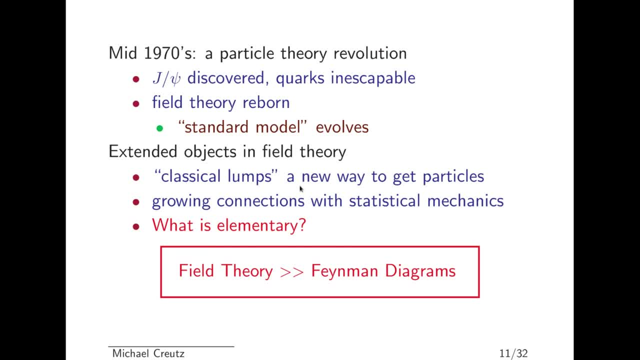 But again, with the extended objects, what is elementary, What we kind of learned at this time was that quantum field theory was really much deeper than just Feynman diagrams. You couldn't see the confinement, you couldn't see these extended lumps, etc. So you had to do something new. 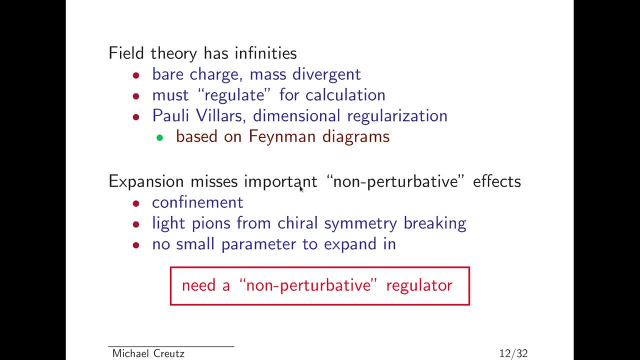 And what made it tricky was, we all know field theory has divergences. The bare mass and the charge are divergent quantities which you have to regulate in some way, And the regulators that were mostly around, such as polyvalar or dimensional, 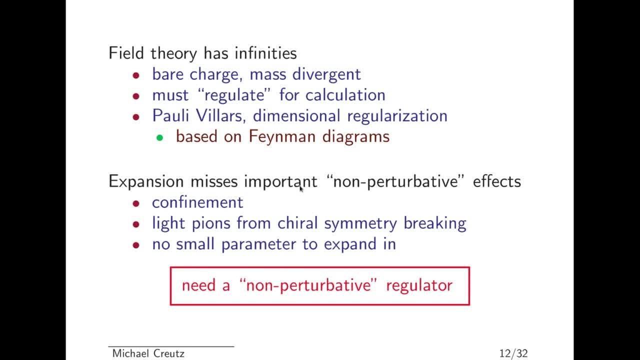 regularization were really based on Feynman diagrams. You would start calculating, you'd come across a diagram which diverged and then you'd have to cut it off. But this idea that you only work with Feynman diagrams misses these non-perturbative effects of 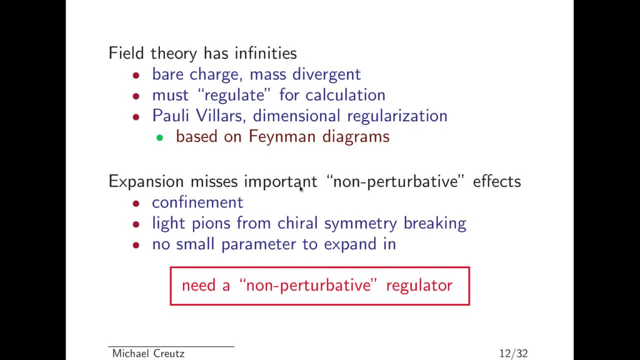 confinement, the fact that the pines are very light from chiral symmetry breaking and there really is no small parameter to expand in. So we need a non-perturbative effect, We need a non-perturbative regulator. This is where 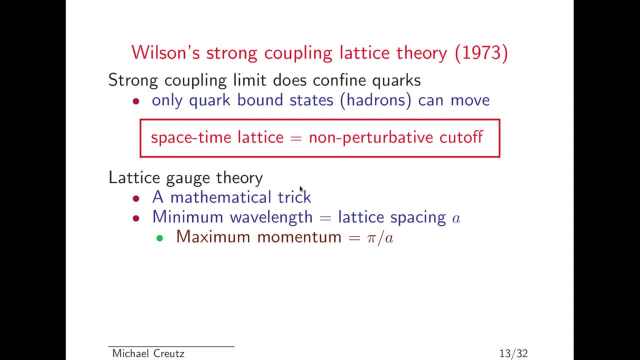 Wilson's strong coupling lattice gauge theory came in. First of all he formulated gauge fields on a lattice and showed that in the strong coupling limit it really does confine quarks. Only bound states of quarks could move. Everything else was just stuck. But what was gradually realized with 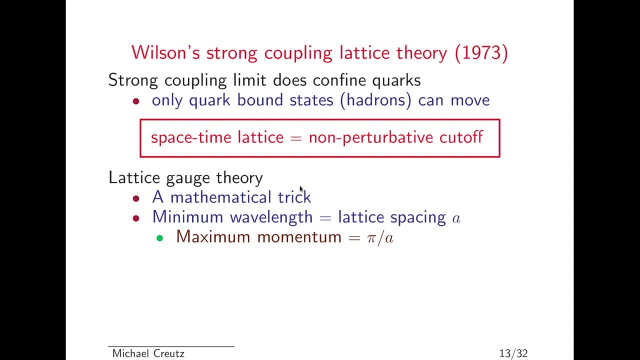 time is that this space-time lattice really was nothing but a non-perturbative cutoff. It wasn't based on perturbation theory And this was lattice gauge theory. Now, I repeat: lattice gauge theory is just a mathematical trick. It's a minimum wavelength A lattice. 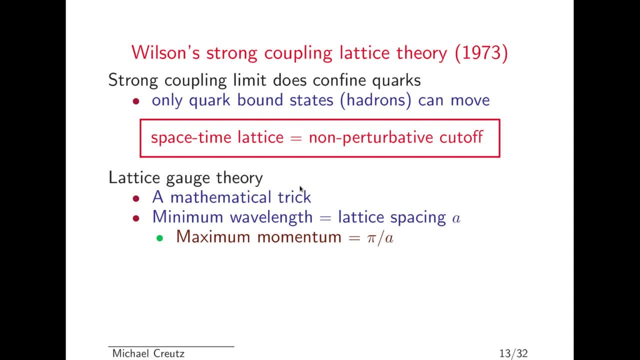 spacing is the minimum wavelength and there's a maximum momentum which is pi over a. So we started realizing we should be discrete and do it on the lattice. Of course, there were a lot of the older people, who would be the ones that die off, who think you should be. 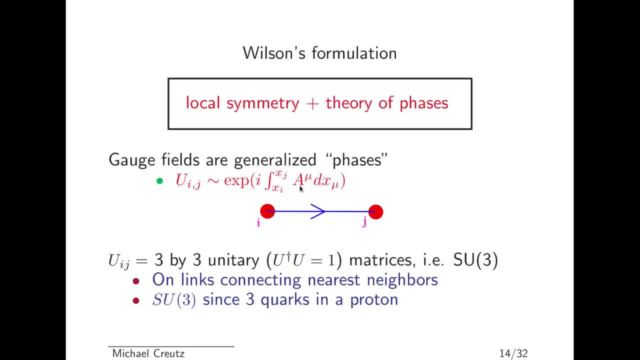 indiscreet and do it continuously. Okay. so Wilson's formulation was really very elegant. It kept a couple of nice features of the non- abelian gauge theory. First of all, it had a local symmetry, which is what non-abelian gauge theory is. 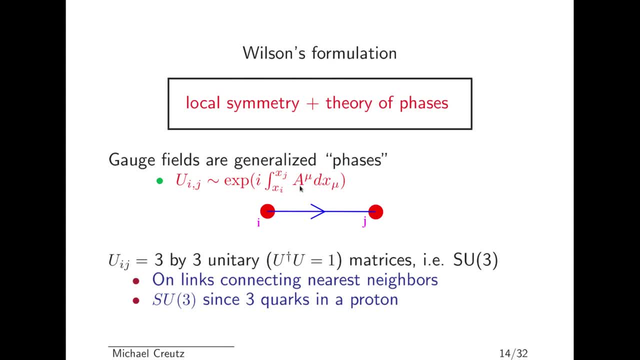 based on, And it was a theory of phases, in the sense that you can describe the interaction of a particle with a gauge field by saying it follows some path and picks up a phase, And so the gauge fields are these generalized phases. And so Wilson said: well, let's. 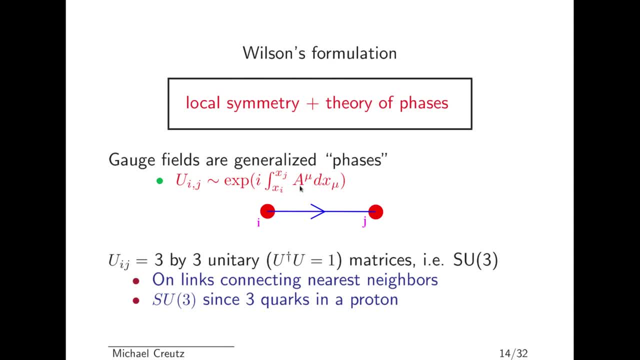 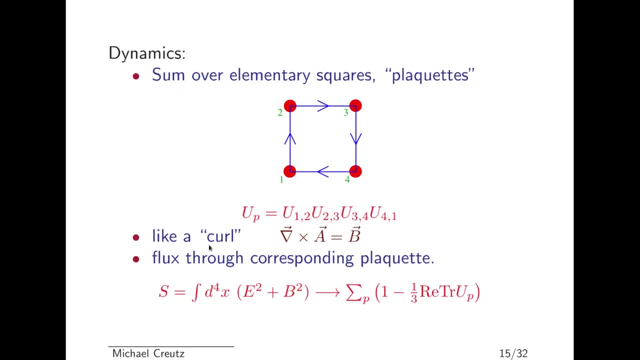 put those on the lattice links. So on any link between some side of i and some side of j, there's this u which is effectively the integral of what the vector potential would be between those two sides. So these u's- because it's an SU3, are three by: 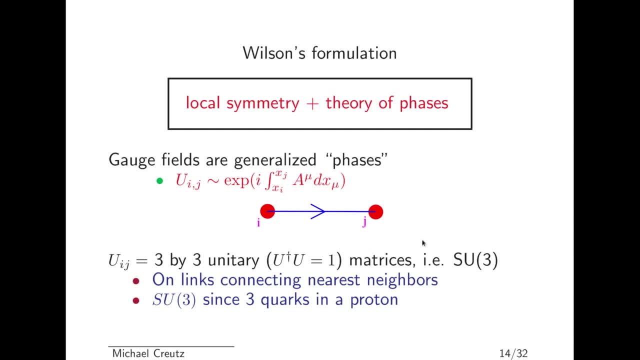 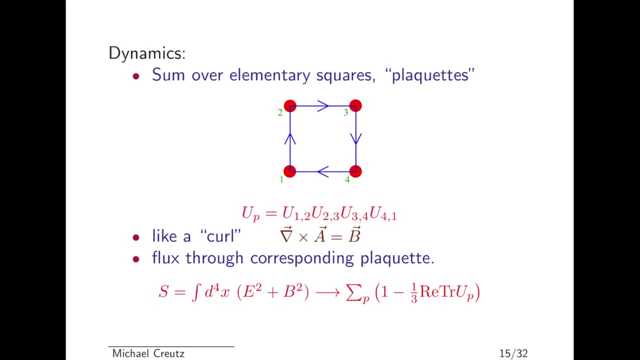 three unitary matrices, which is SU3. And they're located on the links connecting nearest neighbors. And the reason it's SU3 is because this is the way you can form a singlet out of three quarks and make the proton. Now we need some dynamics. We've got our variables. 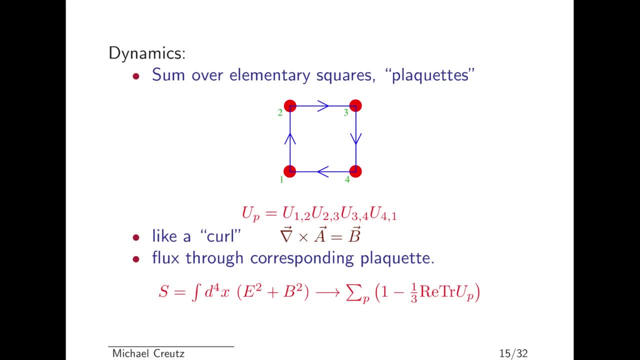 The way Wilson said you could get out of dynamics was to look at elementary squares, which are called plaquettes. You find an elementary square in your lattice. You run around it. This looks very much like a curl And we know the curl of the vector potential. 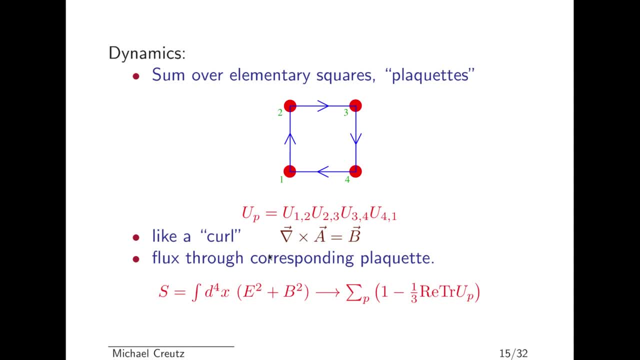 is the magnetic field. So this is a way of getting the magnetic field, And so you use these plaquettes to generate your action. Your action, which is e squared plus b squared, is replaced by 1 minus the product of these u's around. 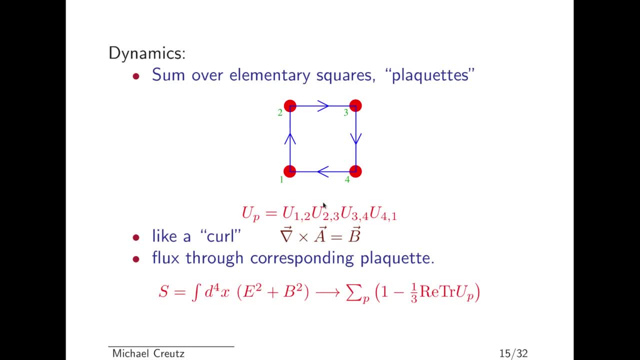 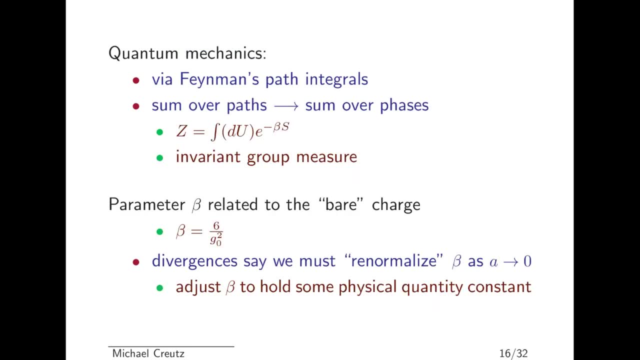 the plaquette e corresponds to time plaquettes which have one time direction, and b is only space directions. OK, so we got our variables, We got an action. Now we wanted to do quantum mechanics. It's done by a path, integral, And for this theory, 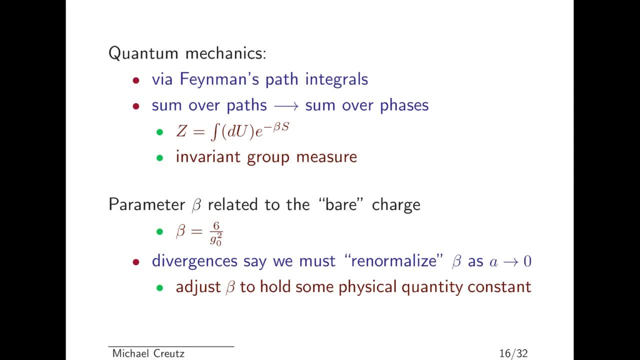 the sum over paths becomes just the sum over all these variables. So we're going to take either minus our action and integrate it over everything around, which is all these u's. This is also elegant because there's a very natural measure when your variables are group elements. 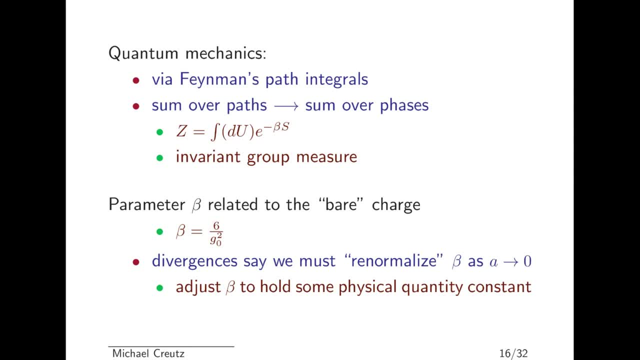 This is the Haar measure, And when you do this, the parameter beta, you can show that it's related to the bare charge of the mass theory. beta is proportional to 6 over g squared. Now again, this is supposed to be a renormalizable field theory. 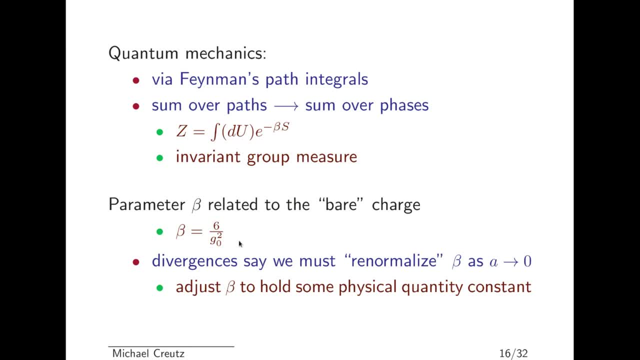 And renormalizable field theories have divergences so we have to renormalize it. We must normalize beta as we take the lattice spacing to 0. So the basic idea is to adjust beta as you vary the lattice spacing to hold some physical quantity constant. 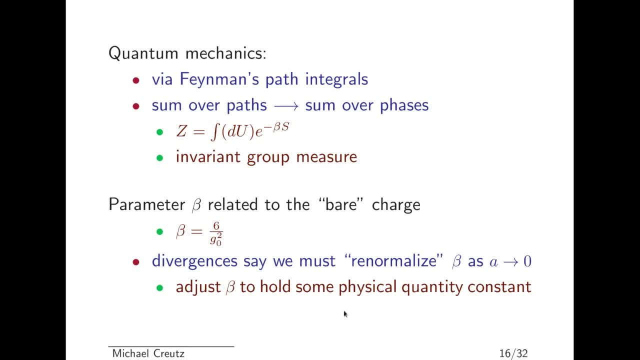 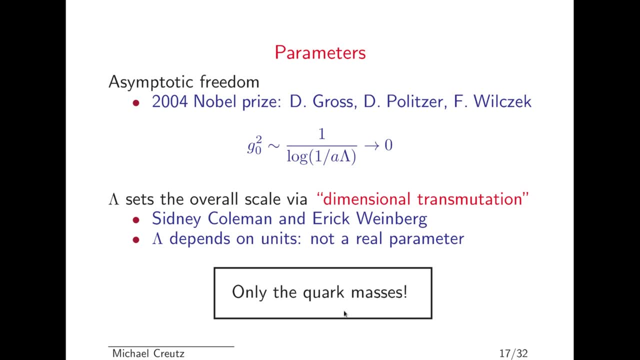 Oops, Yeah. Now this theory is very nice and it's got a real scarcity of parameters Because of this asymptotic freedom thing which goes to what did? the coupling constant should go to 0 with the lattice spacing. So lattice spacing and its logarithmic. 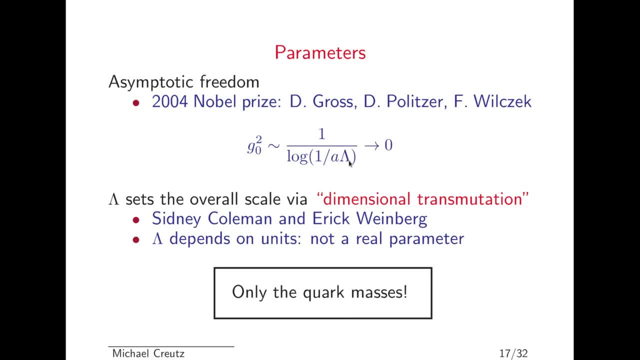 And this requires some kind of overall scale for this decrease in the coupling constant, And it's really kind of cynical At this time. Colman and Eric Weinberg gave this a very nice name. They call it dimensional transmutation. You start with the theory which has a coupling constant. 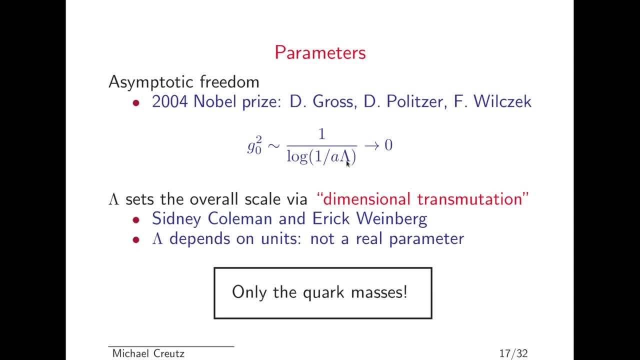 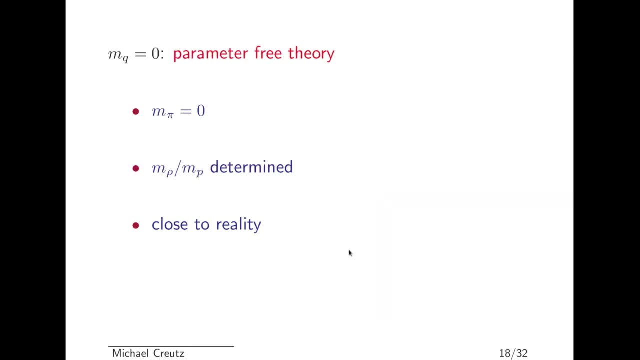 and you replace it with an overall scale. Since it's a scale, it depends on the units you use- MeV or feet, whatever, So it's not really a parameter. The only parameters of this theory are the quark masses. 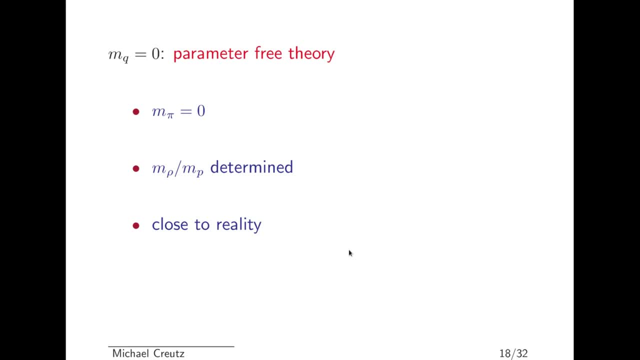 And this raises an interesting limit: turn off the chord masses. we have a theory which has no parameters at all. the pion becomes massless and all the other mass ratios are determined: the ratio of the row to the nucleon. and this isn't too far from reality because the pion is quite light and we'll be discussing that a lot in the 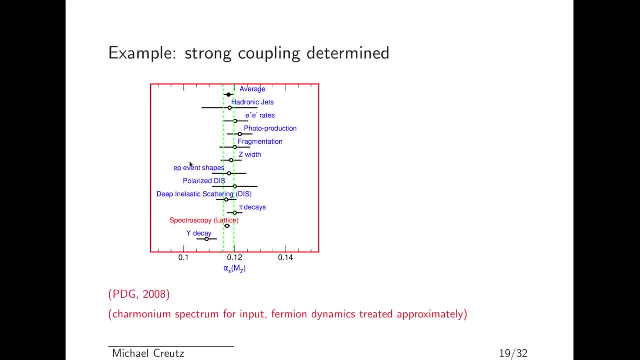 next lecture. so, uh, the strong coupling is not a parameter, it's something which comes out, and so this: we calculate this lambda parameter, which is the scale. it's been done in many, many different experiments and the lattice managed to get itself on this graph. this is a pretty old one graph, but 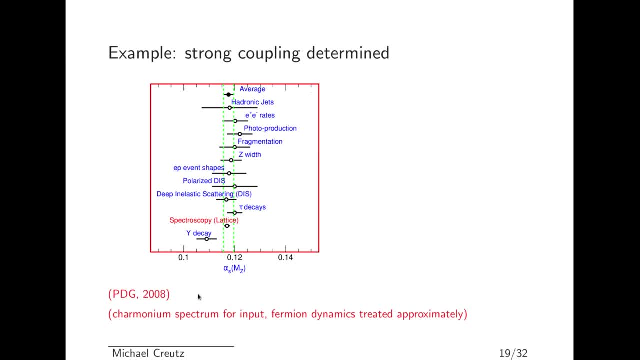 we're still one of some of the best measurements. uh, what they do to do this last thing? you put something in, so they put in the trimonium spectrum. the fermion dynamics is not created exactly here, but it's still pretty good. okay, so this brings us to the idea of numerical simulation. 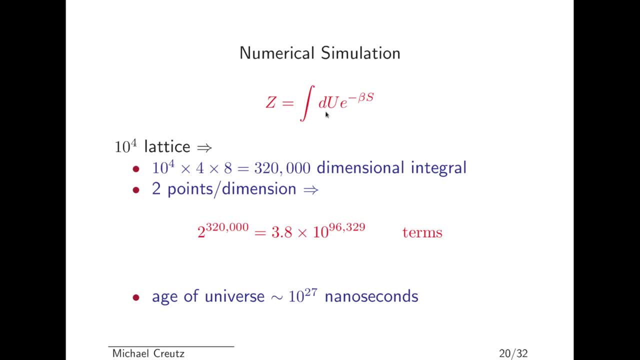 we've got this path integral, which is an integral over all these u's of e to the minus, the action. but this is a very big integral. you could say, well, maybe just just throw it on the computer and integrate it, but it's a big number, a big integral on a 10 to the. 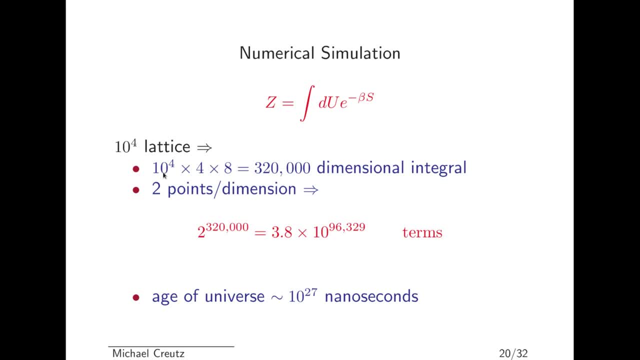 fourth lattice, which is small. these days you've got uh 10 to the fourth times, four links per site, four dimensions, and each link is determined by eight parameters because it's su3, so it's a 320 dimensional, thousand dimensional integral. now, if you just took two points for each of these, 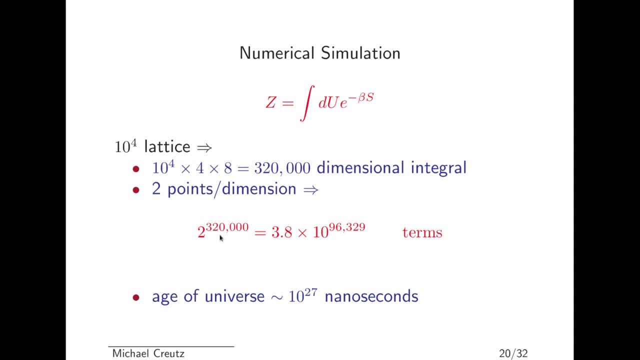 dimensions. you would have to add up to the 320 000 numbers, which is 3.8 times 10 to the 96 329 terms. now this is pretty impractical because you know the age of the universe is only 10 to the 27. 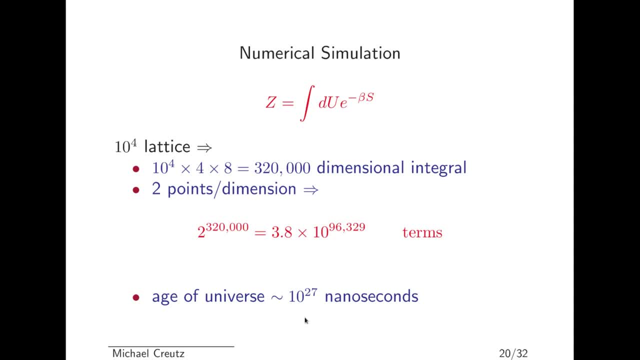 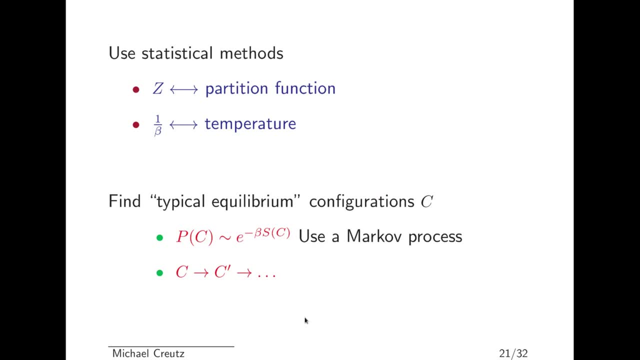 so you'd have to do an awful lot per nanosecond. however, these huge numbers suggest one should use some kind of statistical methods. this formally looks just like a partition function, with one over beta being a temperature, and if you think of statistical systems you're used to, for instance, 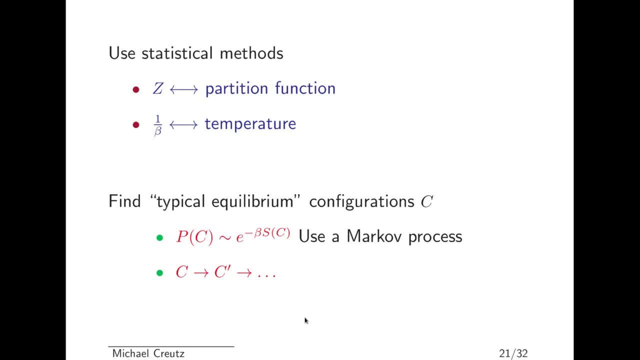 a glass of beer. there are many, many ways you can arrange the carbon hydrogen, nitrogen, et cetera atoms in the beer and it would still be a glass of beer. and you know, you only need about six glasses of beer to know all of its important properties. so that's the idea of the monte carlo we find typical. 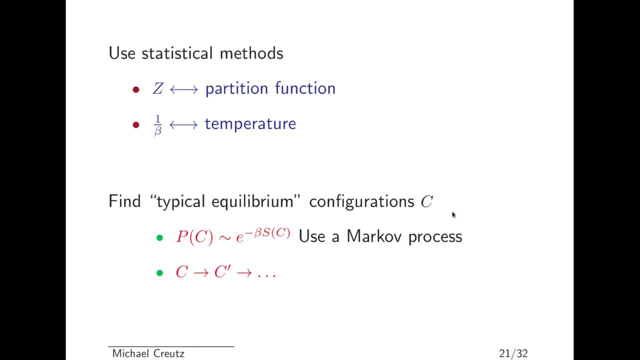 equilibrium configurations. we don't need them all, so we want to generate configurations of the probability given by this, even minus beta times the action. for that we use a markup process, and in these lectures you'll be told lots of detailed ways to do it. but you take a configuration. 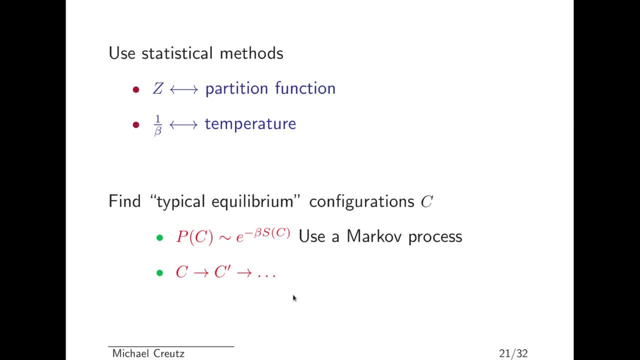 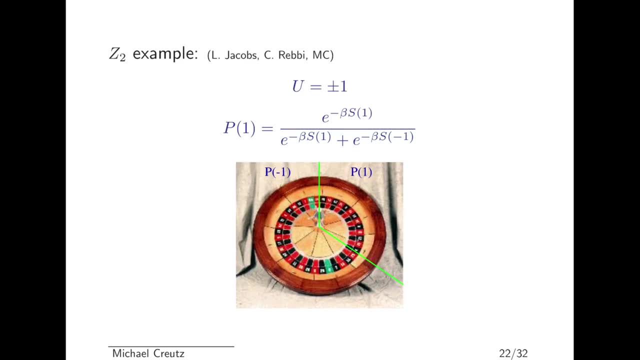 you make a little change, keep making changes and use approach which makes it approach the equilibrium distribution. so, for example, a long time ago we played with a simple model called z2 where the user would just take two values plus or minus one. so what you would do is you would loop over your links and 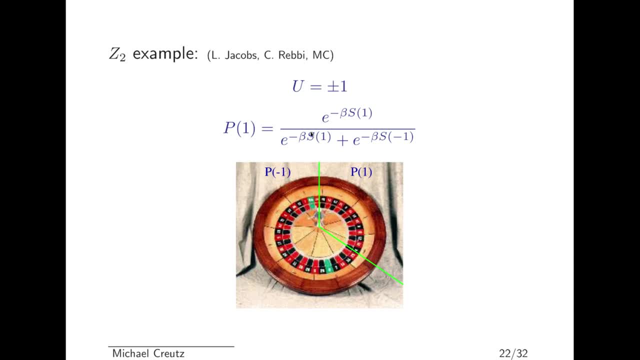 when you come to some particular link, you would calculate the probability. this thing should have the value one and you have to normalize it by the two possibilities you could have. then you take your roulette wheel, spin it around, and which side it ends up on is what you do you. 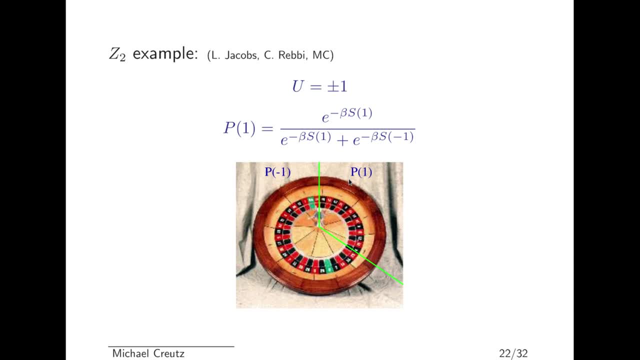 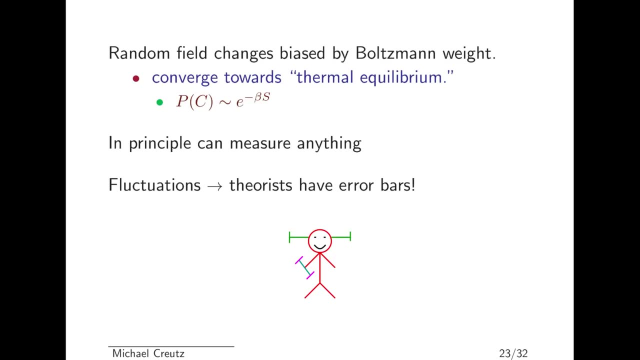 set the link to that number, then you go on to the next link and proceed. so these programs are actually quite simple. uh, you make random fields with changes based by the bolts and weight in such a way that they converge to thermal equilibrium. in principle, this is very seductive because you've got the whole lattice right there in front of you. 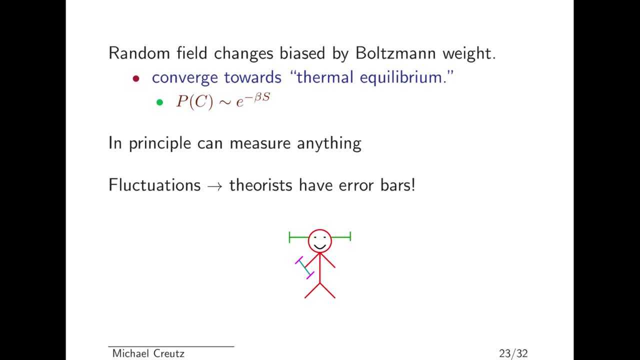 you can, in principle, measure anything you want, but it's only a statistical thing. so are there going to be fluctuations, and so theoretical physicists are not used to having fluctuations, and all of a sudden we've got our little error bars, which is pretty cool. now there are other errors besides fluctuations, very systematic ones, which will be talked about. a 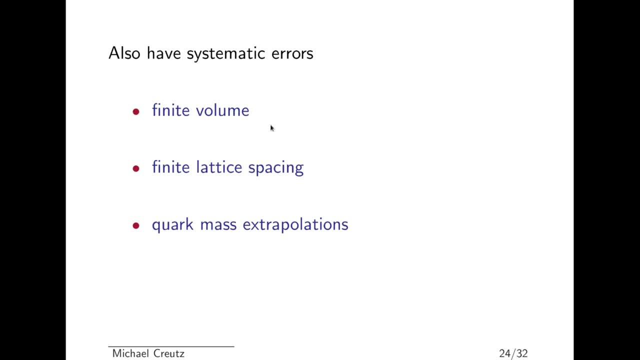 lot of this meeting i guess. first of all, you can't really write kind of infinite lattice because you can only have so many words on your computer. we have to work at a finite lattice spacing. so we have to consider several different lattice spacings and try to do a continuing limit. 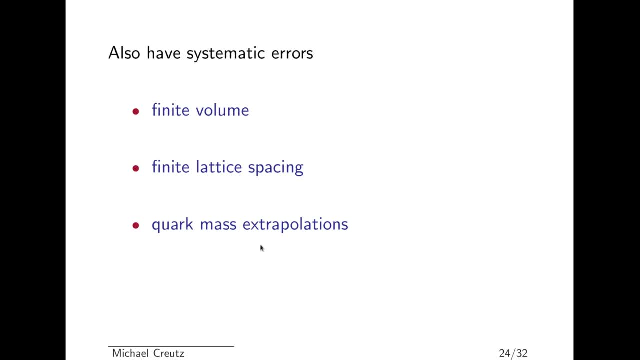 and another problem which is starting to go away now is that as the quarks get really light, the pions get really light and the convergence of these integrals gets very, very slow. so normally quite often people have had to work with quarks heavier than the physical. 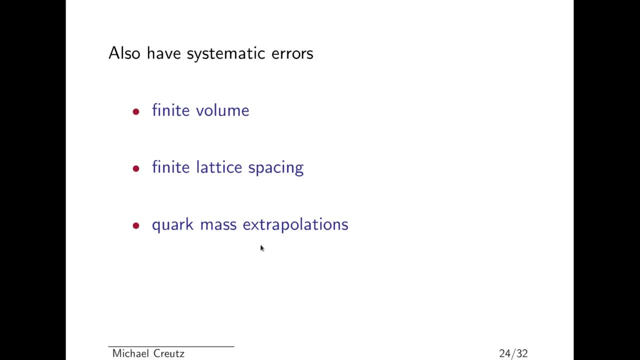 masses, uh, and then try to extrapolate down. so various things have been done over the years. this is an old picture just measuring the inner quark force. you see that it does indeed go to constant large distances, which is the confinement of that. it's also they've done this for several different lattice spacings, which corresponds to: 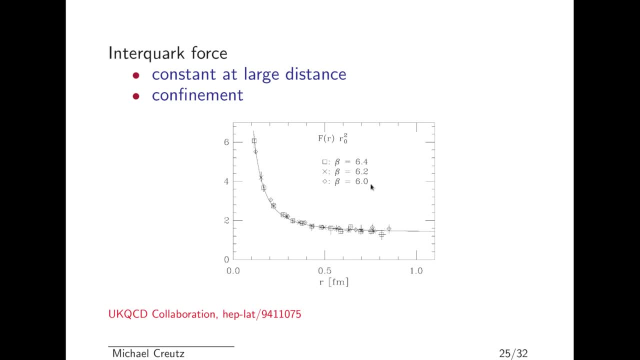 betas, and they all come on top of each other, so you obviously are close enough to the continuum limit. so this is very pretty. uh, this was the uk qcd and this is, i said, a very old paper. okay, now what you want to do is know something about the particle masses. 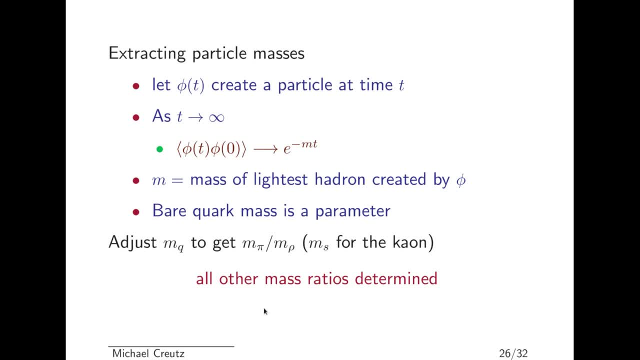 so let's consider some operator which can create a particle at some time: t. as the time is large, you can measure the correlation of this operator at the later time, t, and say t equals zero, and this correlator should fall off as e to the minus the mass. 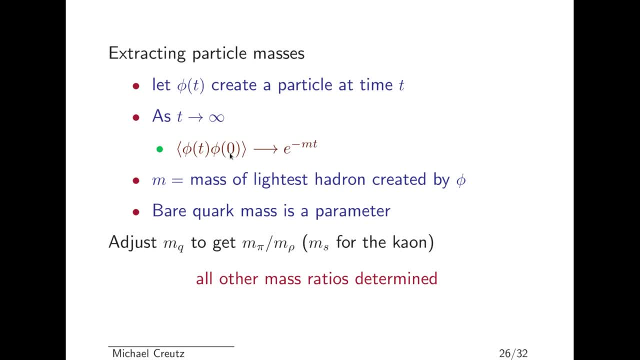 of the lightest hadron which can be created by phi. in this game the bare chord mass is a parameter, and so you have to adjust to chord mass to get something right. it's again a normalization trick. so you, if you, can get the pion to the row right, then you know what the court mass is. 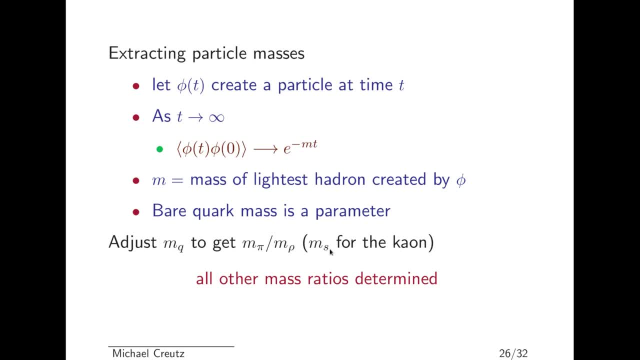 you would. you would adjust, uh, the strange quarter mass to get the can right. once you've done, the pion in the can and the, basically the proton cup, determines the scale. everything else is determined. there's no other parameters. it's amazing. so here's a picture of the spectrum. is: 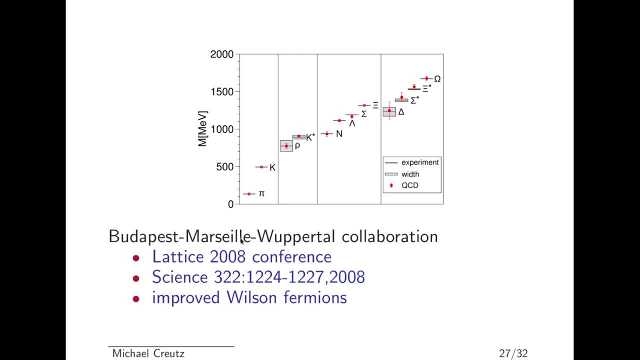 released by the buddha pass from marseille, whoopertal collaboration, a few years ago, and they they had to put in the pion mass, the can mass, and i think the other thing they put in might have been the omega, i'm not sure. anyway, 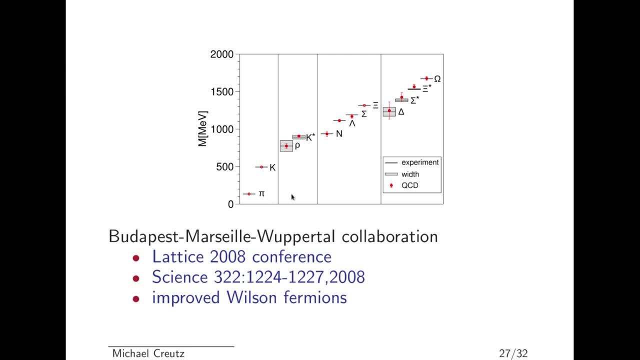 they can be able to calculate the whole spectrum with only a couple things being fixed, and this was done with a particular formulation of fermions, which we will talk about a little bit in the third lecture. now, of course, the nice thing about qcd is you can also have particles which don't. 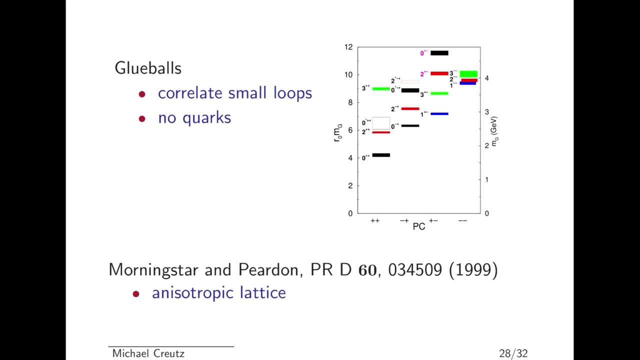 have any quarks. they're basically little loops of flux and these are called glue balls, and morningstar and pierjon went off again on old paper to measure the spectrum and it all comes out very nicely, although the real problem with these things is- and the blue balls mix with 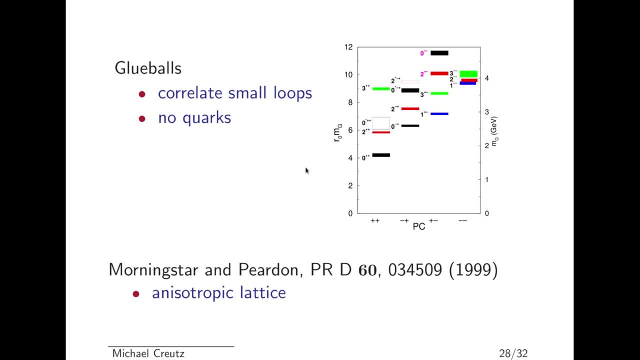 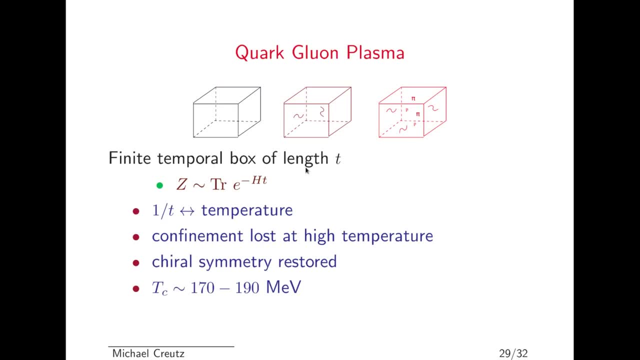 the hadrons containing quarks and that's a very complicated mechanism, but that's a very good line, yeah, subject: Another very popular game in the lattice gauge theory is to measure this thing called the cork glue and plasma, And the idea is that when the vacuum gets really hot, there's a transition. 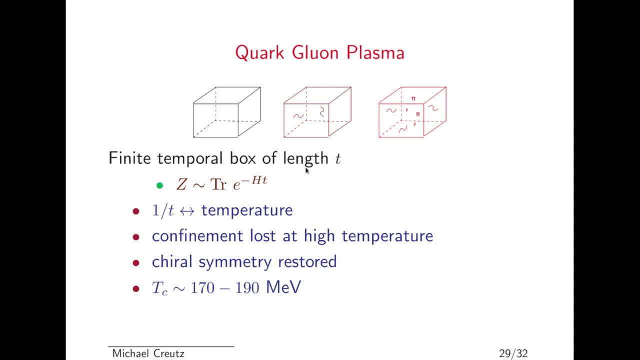 to a new phase in which confinement is lost. Now, what does it mean for a vacuum to have a phase transition? The vacuum is empty. It can't have a phase transition, can it? Well, imagine a box. You take a little box and you make the walls get hot. And when the walls get hot, though. 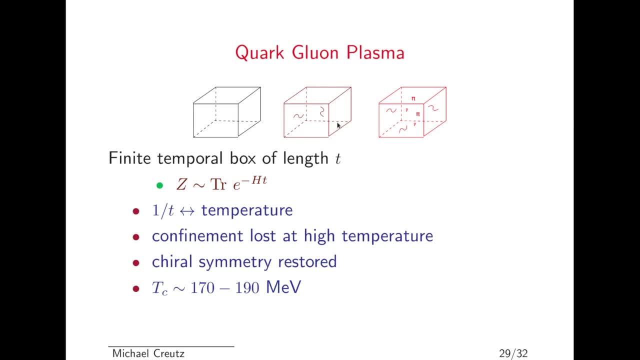 eventually it will start glowing red and hot And the box will have little photons inside it. So it's not really empty anymore. It's got radiation from the walls And if you make it hotter and hotter and hotter, eventually it fills up with protons and pions and all the other. 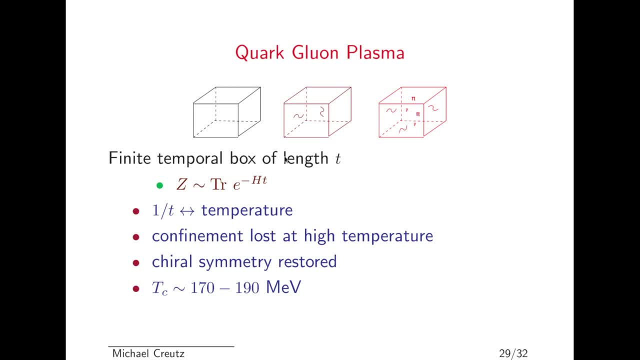 particles, just a thermal mixture of them, And in fact the partition function is formally the trace of either, let's say, Hamiltonian times, time, where time is the size of the box, which is and plays the role of temperature. So it's been observed that confinement is in fact 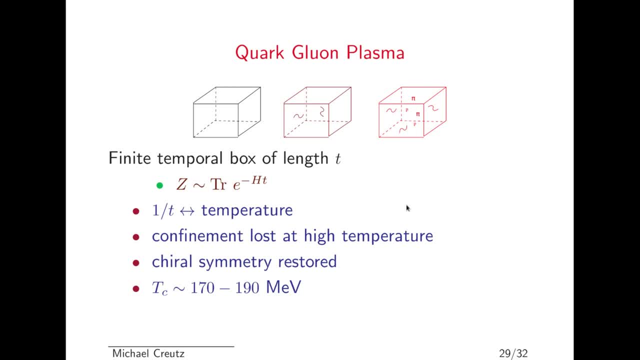 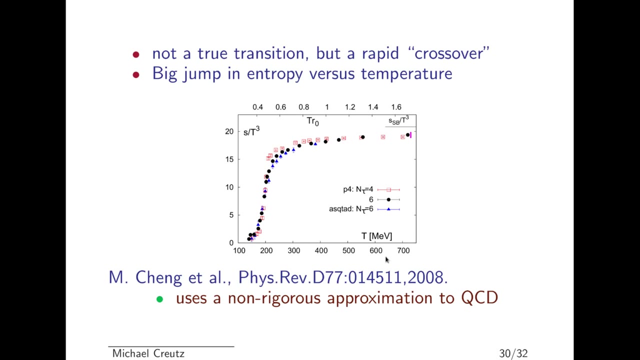 lost at high temperature and chiral symmetry gets restored. This may not be the latest number, but it's somewhere in the range of 170, 190 MeV where this happens. It's not a true transition, It's just a very rapid change in behavior. Here's a measure again an old paper, The 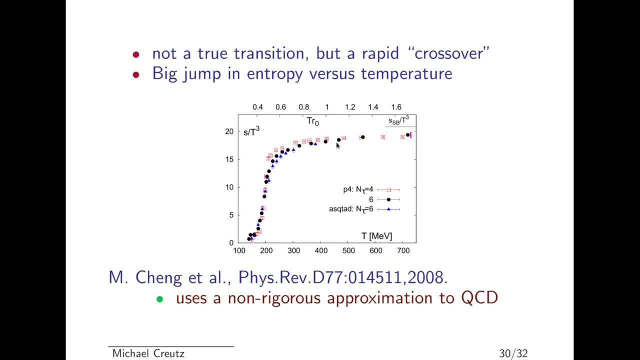 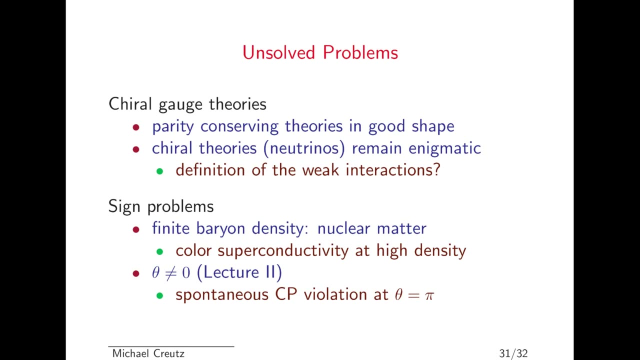 very narrow range of temperature. Now, this particular calculation is again using a non-rigorous approximation, but it's a pretty good approximation, Okay. so this is the basic structure of lattice gauge theory. There are some very interesting problems which are unsolved, Parodic and preserving theories like the strong interactions. 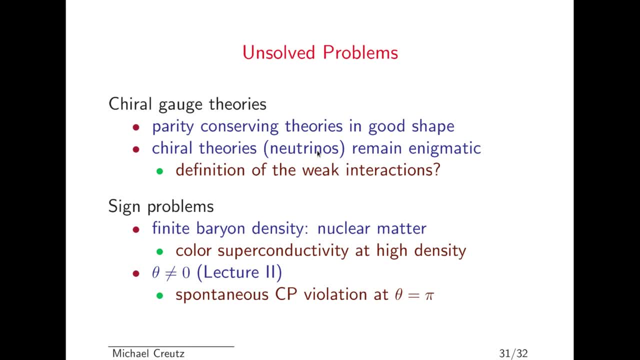 are in good shape. But chiral theories like the theory of neutrinos, which are only left-handed, we really don't know how to do that on the lattice. And because we don't know how to do it on the lattice, if we're using the lattice as a definition of field theory, do we really? 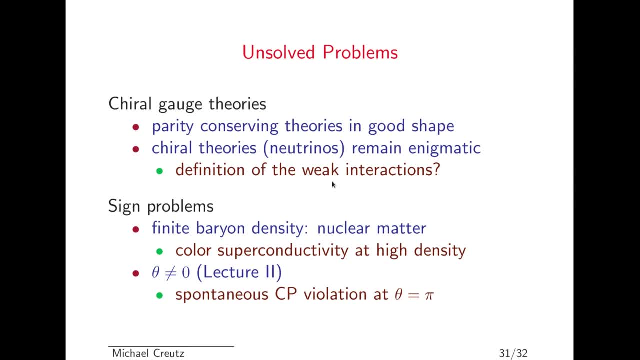 have a decent definition of weak interactions. This is a sort of a standing problem for a long, long time. There's another problem which is more of a technical one. We've assumed we're doing weights by the action. but if the action is not real, then the weights can. 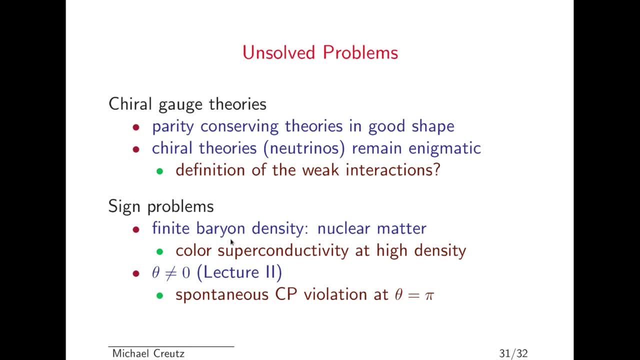 be complex numbers And this occurs at finite variant density, which is very important because you want to understand nuclear matter, which is in a finite density, And we believe there's a color superconductive phase at very high density, but we don't know how to study that using 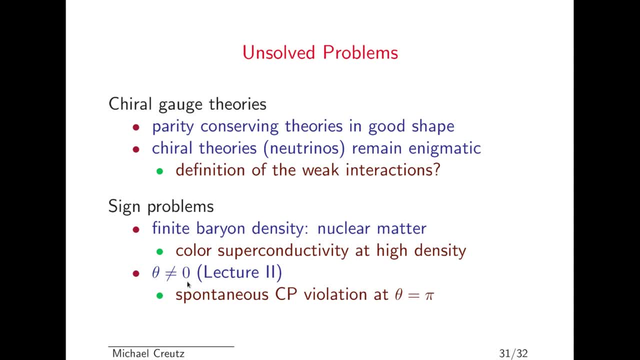 lattice techniques. There's a parameter in QCD, which I'll get into in the next lecture, called theta, And when theta is non-zero, there's again sign problems. And this is: you're missing some interesting physics here, because it turns out when this: